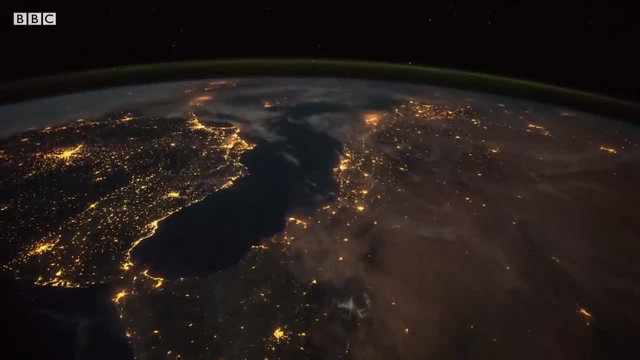 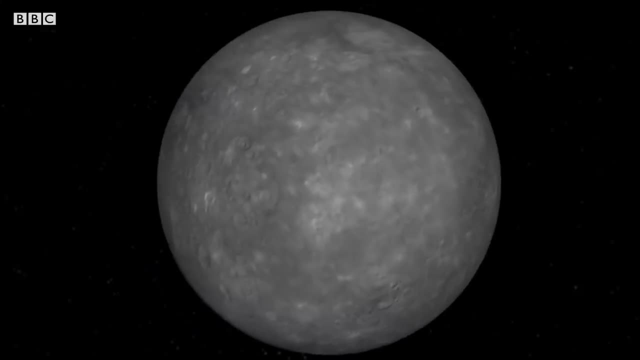 the layer of gas that surrounds a planet. So, for example, Earth's atmosphere is made of nitrogen, oxygen, argon and a little bit of water vapor as well. The planet Mercury and our Moon. on the other hand, they don't have an atmosphere, hence why they look like. 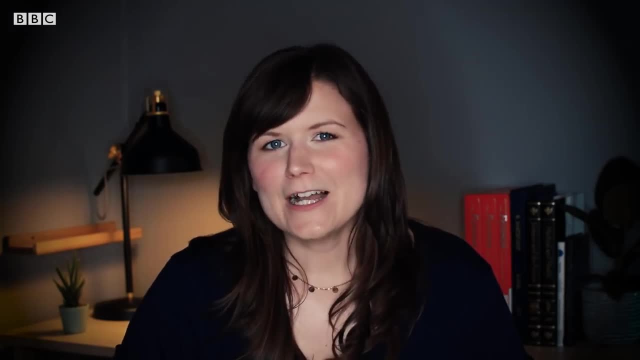 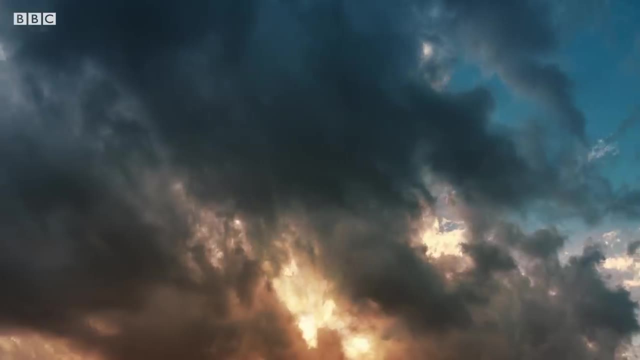 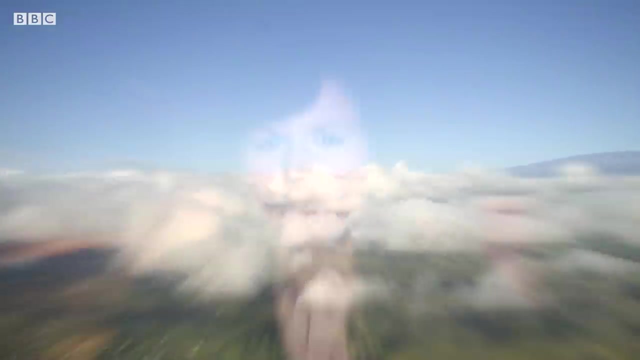 grey, lifeless rocks On Earth. a cloud forms where it's too cold for water to stay as a vapor in the air. Now, that can happen with other materials too, just at different temperatures. so it's essentially possible to have a cloud made of anything. But what about planets that are so hot that things that exist as solids on Earth are actually liquids and gases in their atmospheres. I'm talking about things like rock and lava. Imagine it being so hot that lava evaporates into the air, forming clouds, and then you get lava raining from the sky. 55 Cancri E. 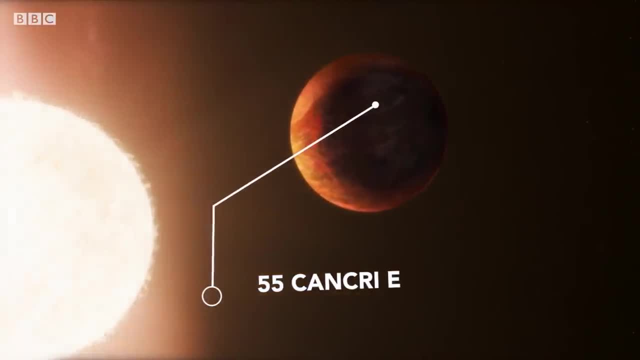 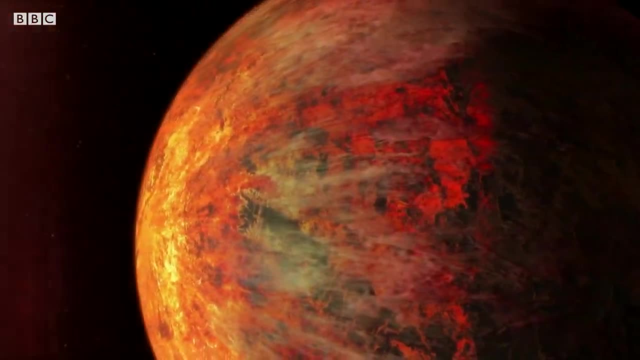 is an exoplanet that's about 40 light-years away from us. It also has the largest atmosphere possible On Earth: it's about 20 times more orbits really close to its star. Not only that, it's also tidally locked, which means 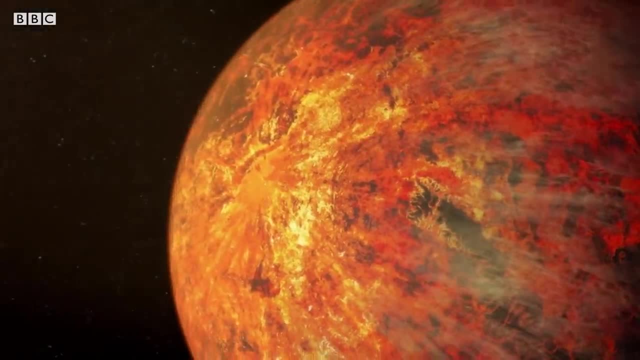 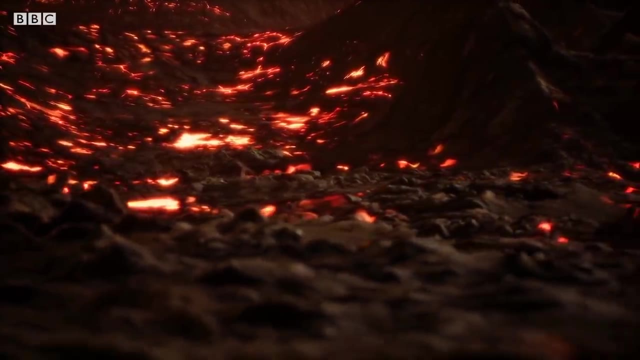 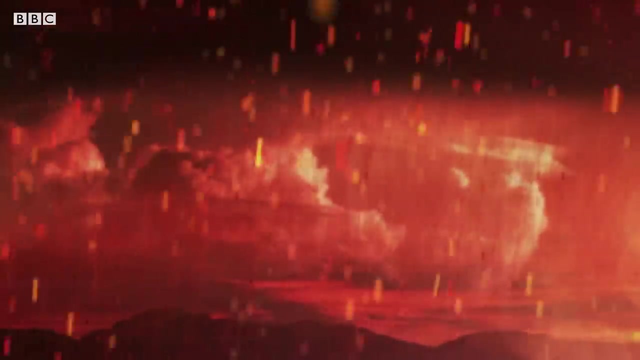 that one side of the planet always faces its sun and it's always daytime there and it's boiling hot. The day side is permanently covered in an ocean of molten lava. It can be hard to picture what lava rain would actually look like, but volcanic eruptions. 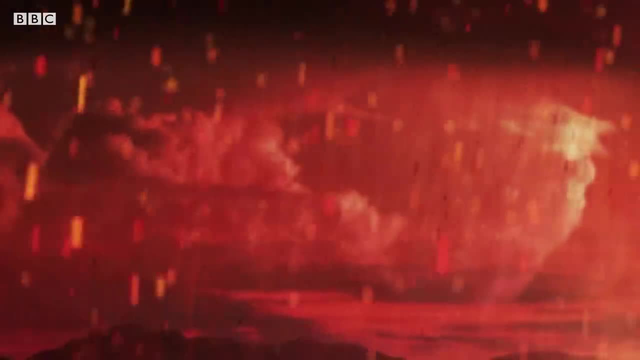 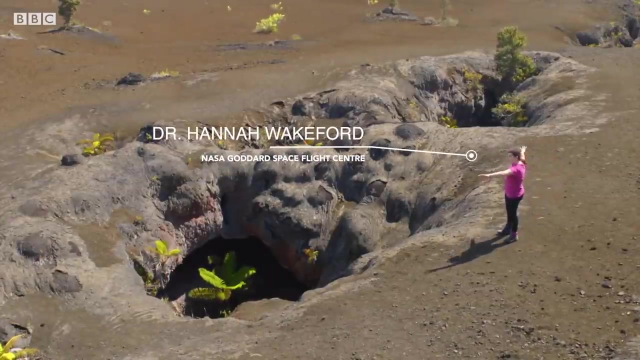 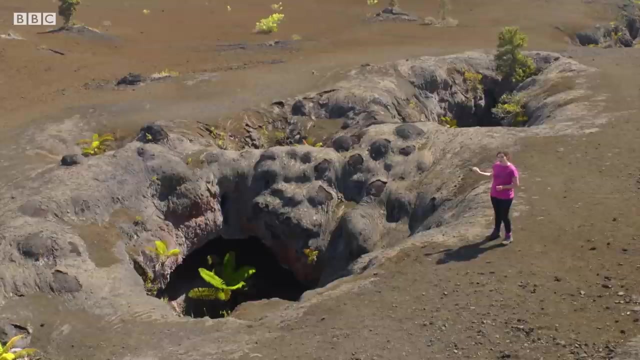 here on Earth in places like Hawaii. give us a hint of what it might look like. Right here was the site of a massive eruption. All along this fissure, fountains of lava shot into the air nearly 100 metres high. The liquid lava droplets then cooled and solidified. 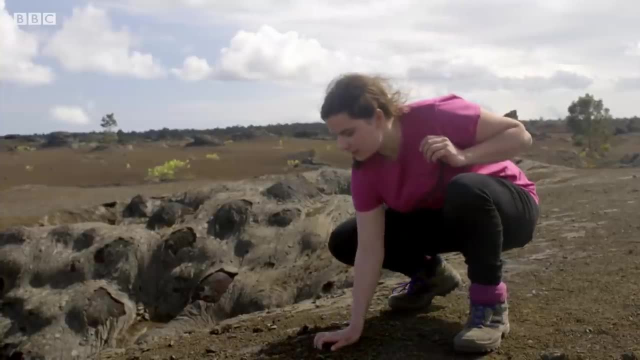 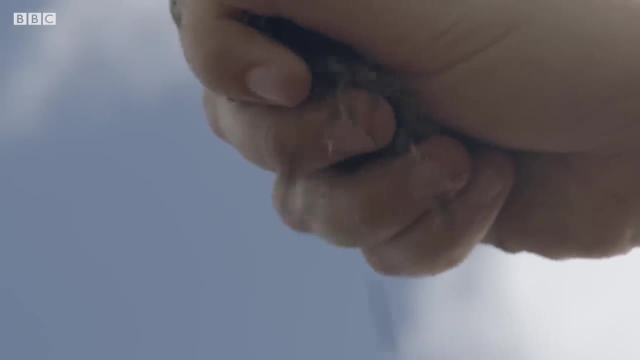 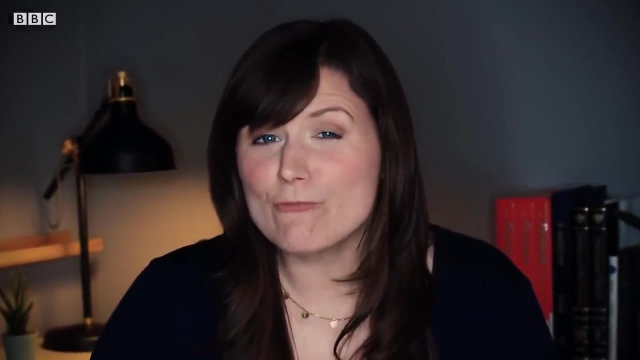 in the air before raining down onto the surface as these tiny pebbles. This is what we think the rain might be like on planets like the 55 Cancri e. Planet hunters and astronomers think they have found an exoplanet with the strangest. 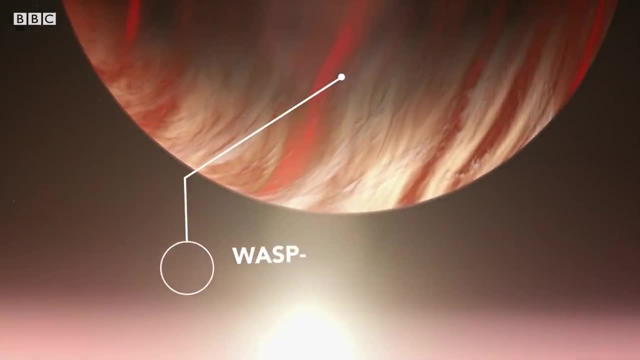 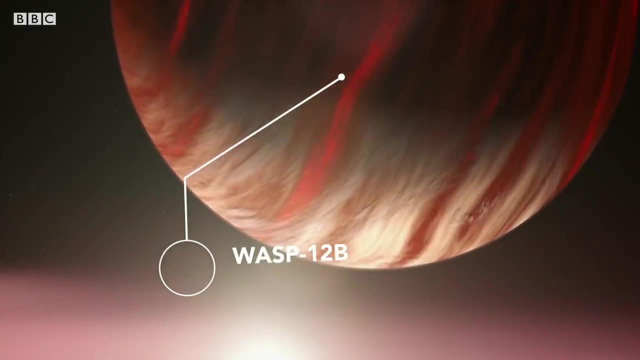 rain in the universe. WASP-12b is an exoplanet 12,000 light years away. It's a gas giant like Jupiter, but it's twice as big and its atmosphere is 2,000 degrees hot In an atmosphere. 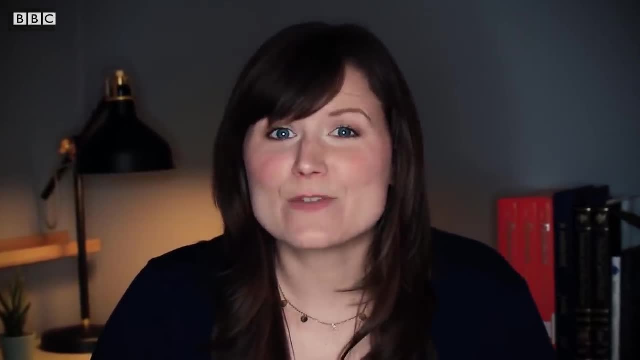 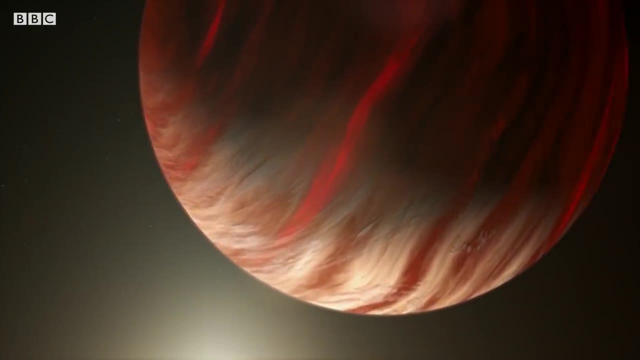 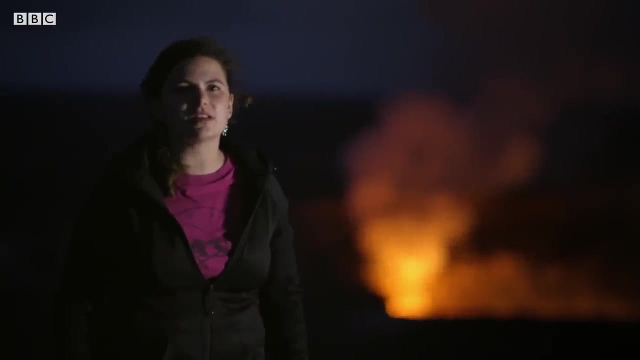 like that, we think the conditions would be just right to give us molten ruby rain, And the way that it scatters light suggests that there are clouds high up in the atmosphere. At this part of the atmosphere, the temperature is around 2,000 degrees, so the most likely substance forming these clouds is an aluminium. 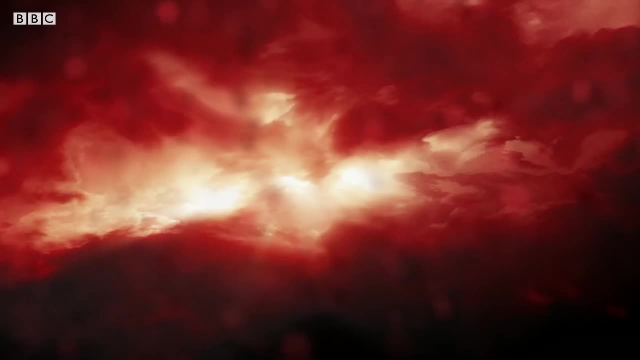 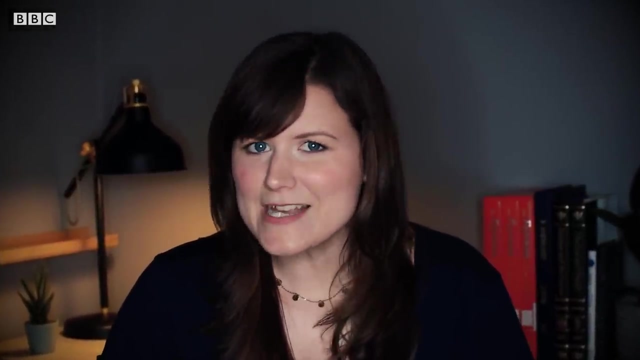 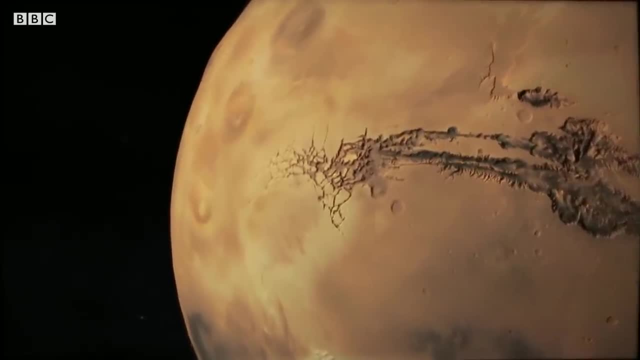 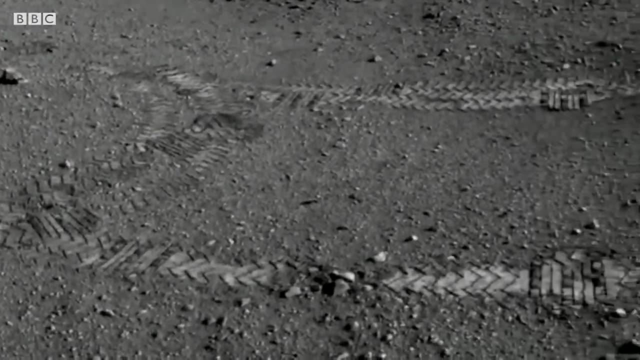 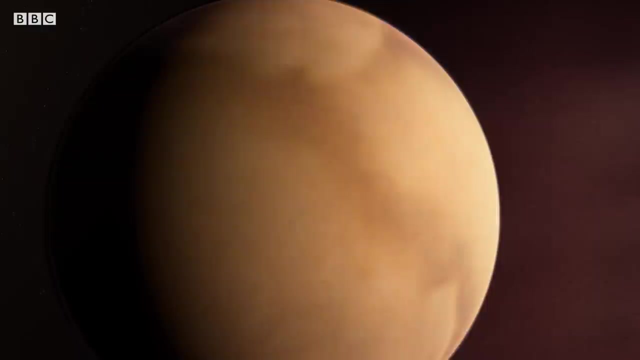 really low atmospheric pressure on Mars means that it can't trap any of its heat. So Mars is a cold, barren desert compared to Earth or to Venus. storms are so bad on mars that every few years or so they engulf the planet for months at a time. 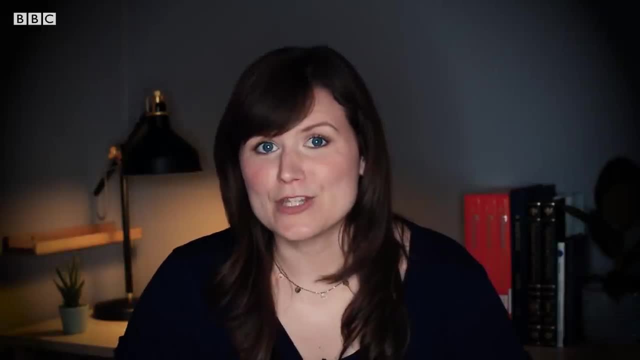 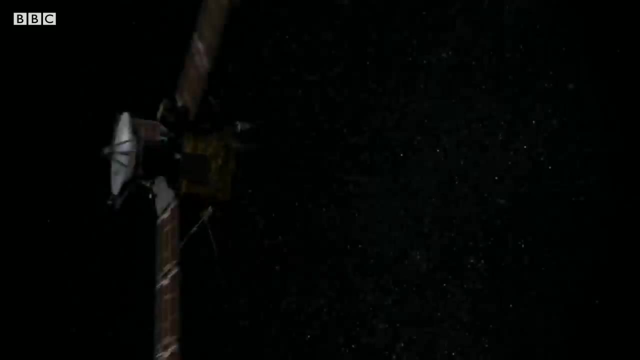 that's going to have a major impact on any future human missions that we send to mars. these storms on mars, though, are minuscule in comparison to what's been observed elsewhere in the solar system. we've sent probes and satellites to all of the gas giants and found 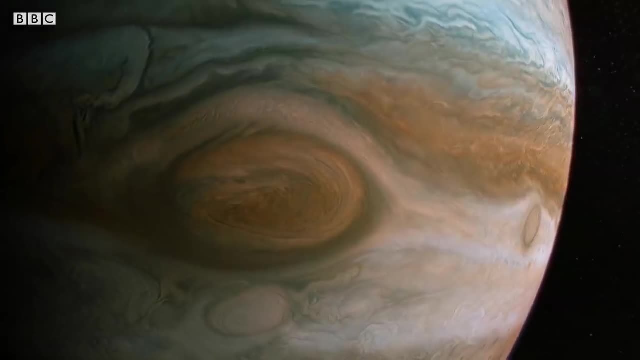 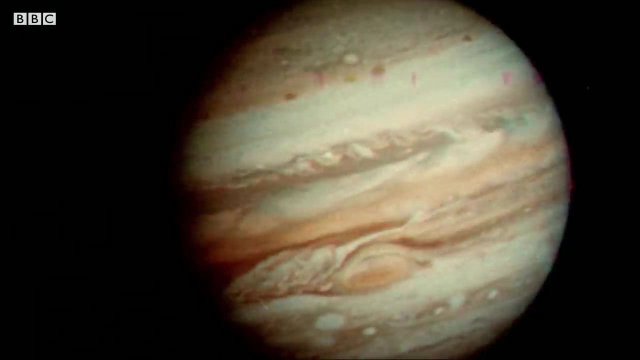 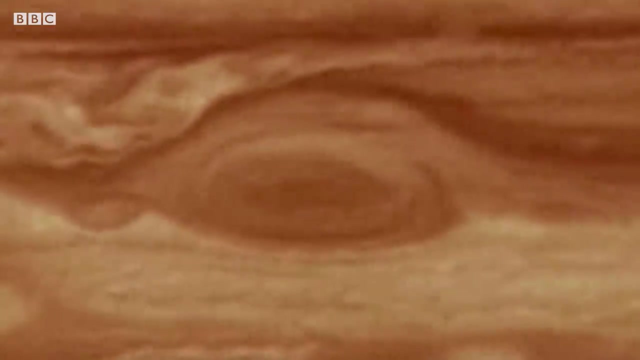 some mind-blowing weather activity. the great red spot is a storm on jupiter that is twice the size of the entire earth. it was first spotted by giovanni cassini through a telescope in 1665, which means it's been raging non-stop for at least 350 years. that makes it the longest living storm. 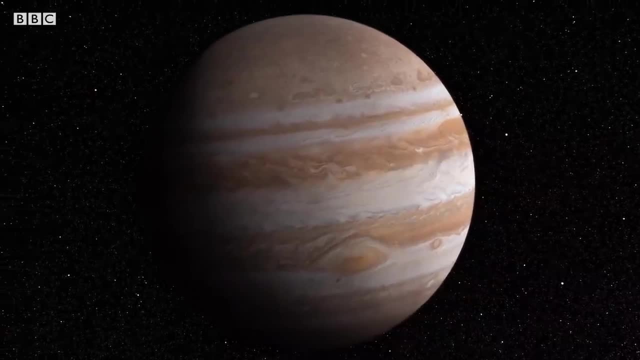 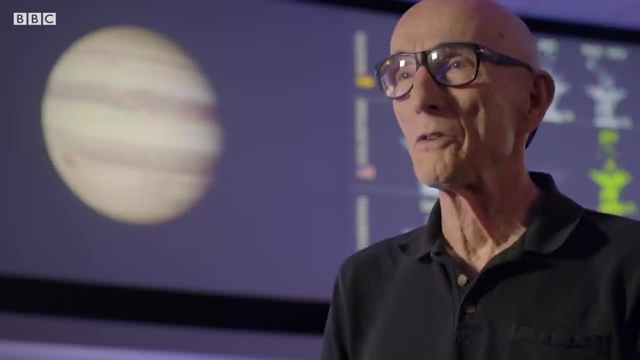 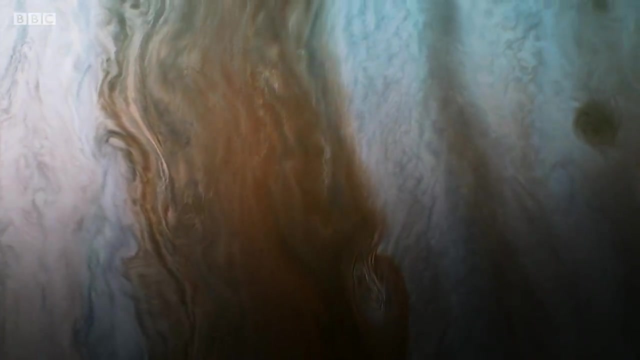 that we know of the outer planets are big balls of gas and that makes a huge difference in the weather, because you don't have continents, you don't have mountains for the winds to rub against and there's nothing to control the weather, the way the continents partly control our weather. saturn is the planet with the largest and most powerful storm in the solar system, covering four billion square kilometers, and we know about it because we've seen satellite images of it growing. on december 5th 2010, the radio receiver on cassini started picking up.